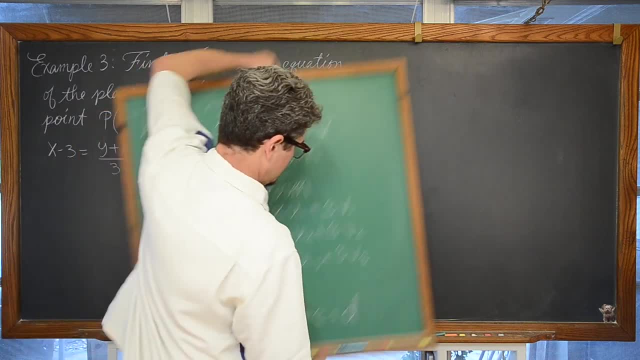 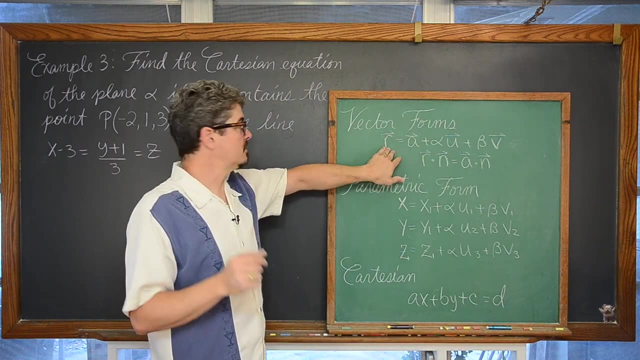 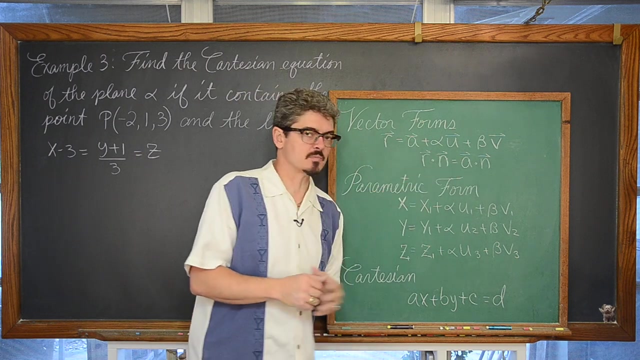 you are going to go into Cartesian form or not. you need a point on the plane whether you are going to use this form or this form. for the equation of a plane in vector format, You need a point on the plane described with this position vector, and you need some kind. 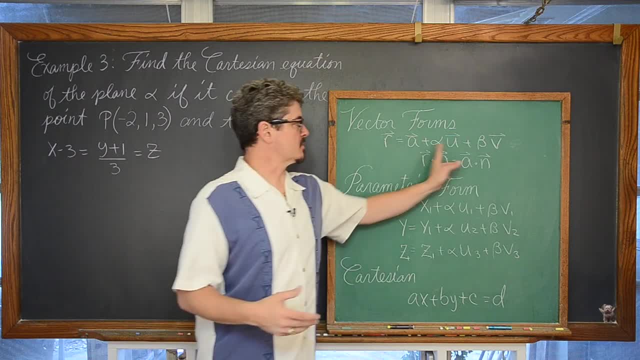 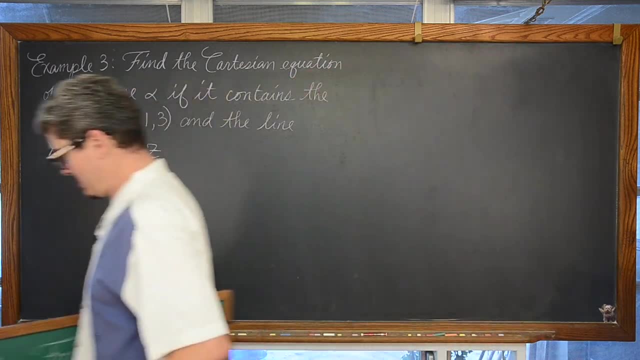 of gradient. The gradient is two vectors, The sum of two vectors which are parallel to the plane, or you are using a vector which is orthogonal. We are going to do the orthogonal one in this video, since we just got done. doingwell, we used both methods in our last example, but 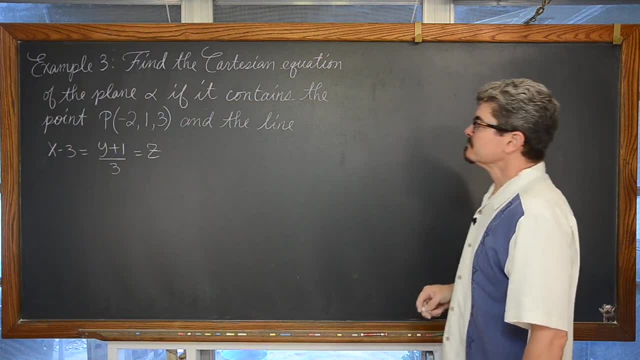 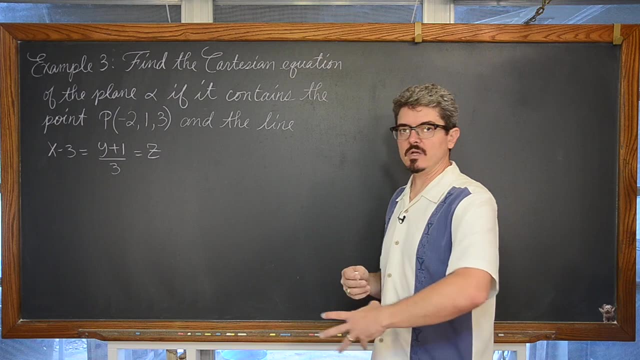 I focused on the one where we used the parallel vectors, or we used the first form. So we are going to write thiswe are going to break this, apart from Cartesian, into the three parametric forms, or that combination of those three parametric equations making up or describing this line. 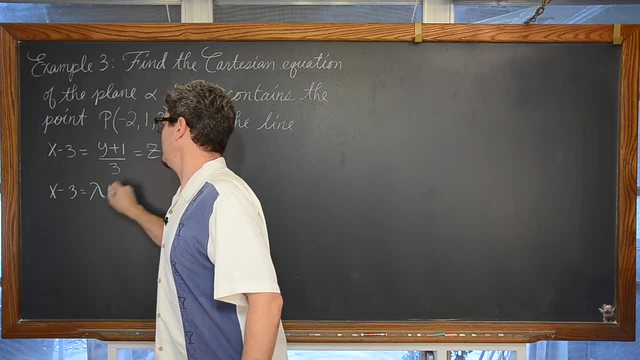 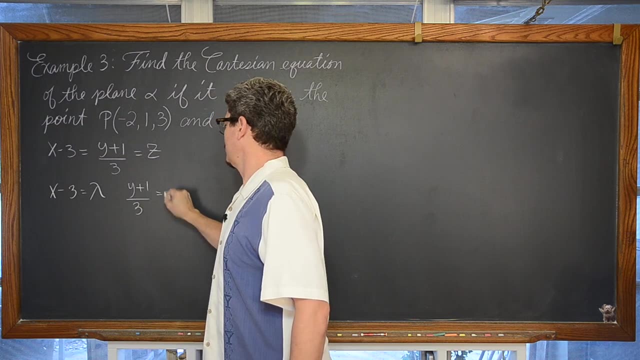 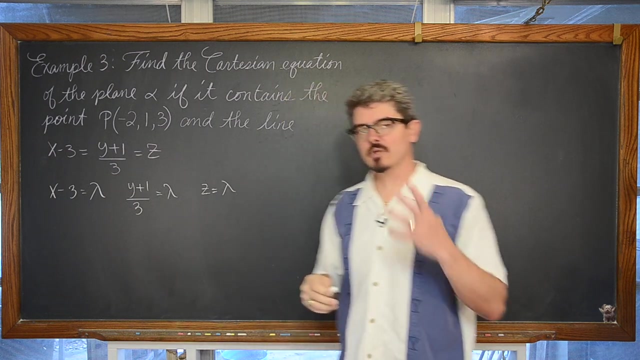 We have x minus 3 is equal to lambda. we have y plus I over 3 is equal to lambda, and we have that z is equal to lambda. Just to make this really, really clear, We are going to make each one of these look identical so we can clearly see what- at least one point- We 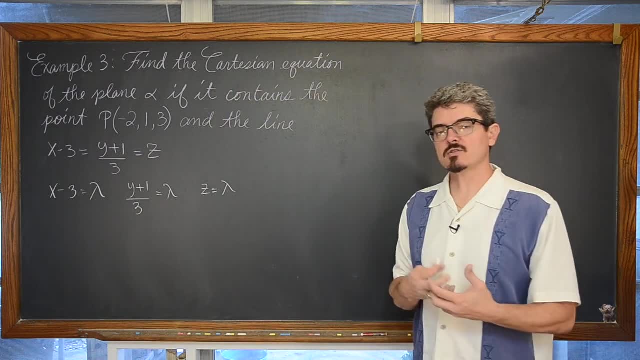 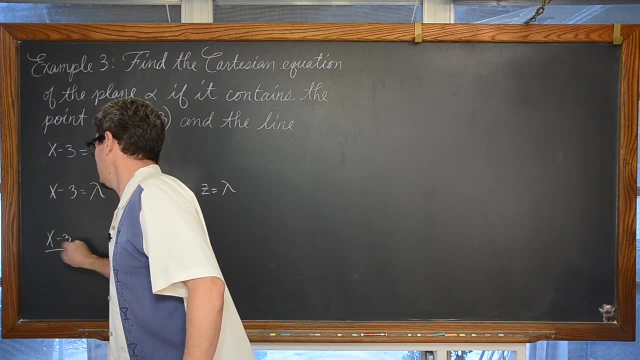 can find one point along this line very, very easily and then find a direction vector or sort of a gradient. Subtitles by the Amaraorg community for that line. So we are going to write this as x minus three over one. We got this already. 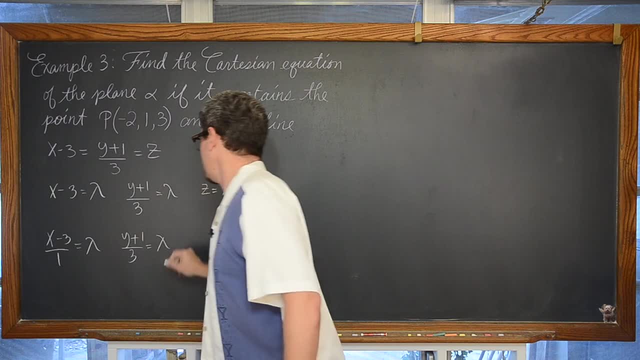 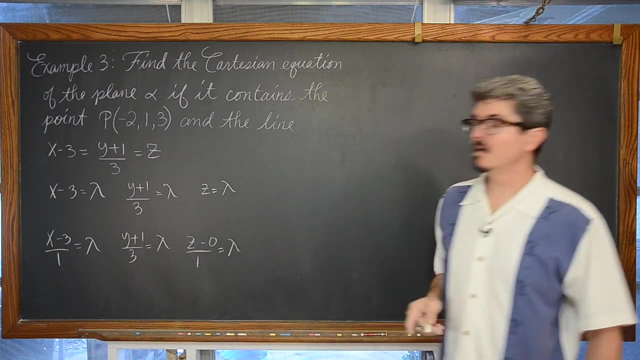 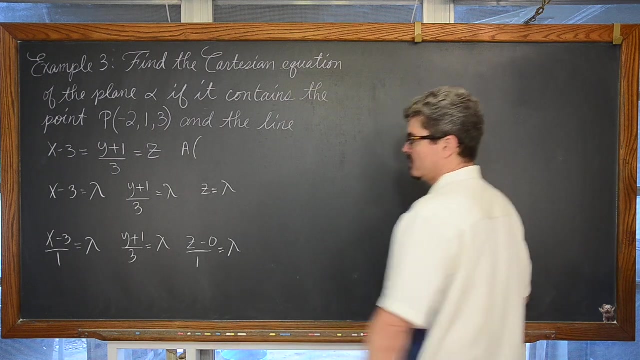 really good. Y plus one over three again is equal to lambda. Here we are going to write that z minus zero over one is equal to lambda. So we can see that the line that they gave us has a point. let's just call it a which has the coordinates of three negative one. 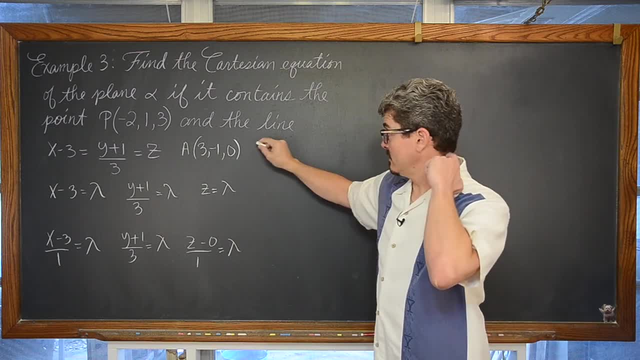 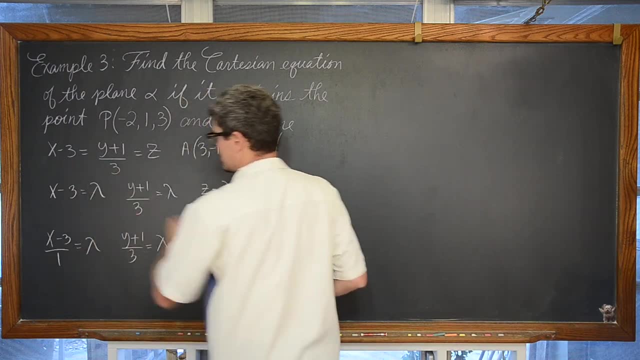 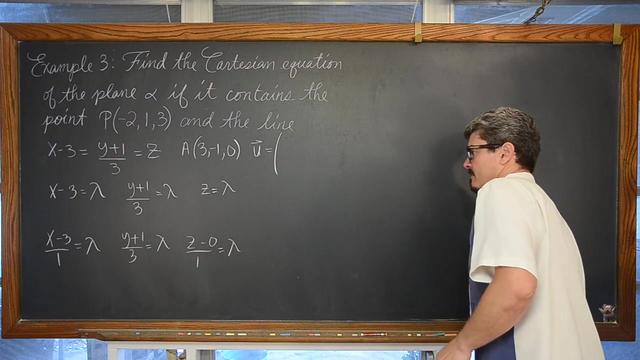 zero and a directional vector, a gradient if you will, for this line is in the denominator Or we can see itactually. I could have done that. I could have multiplied this by three and then subtracted one. I will show you that as well. I will just do it on. here We are. 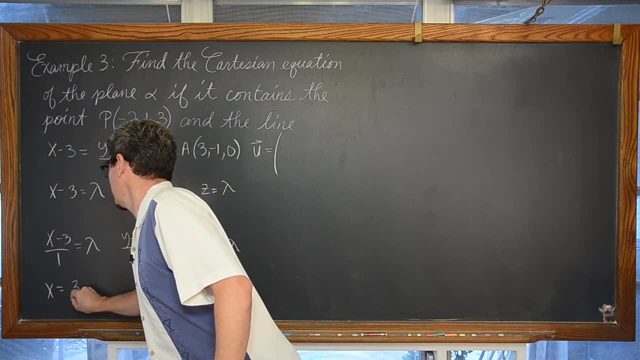 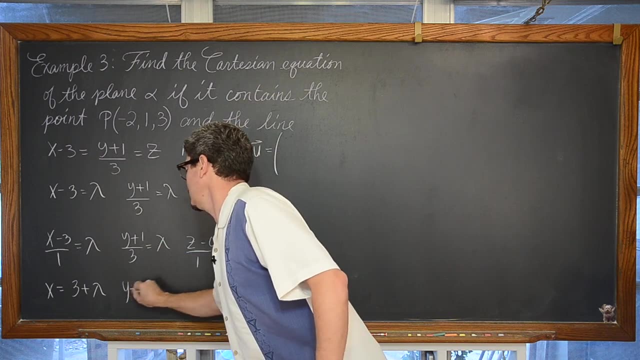 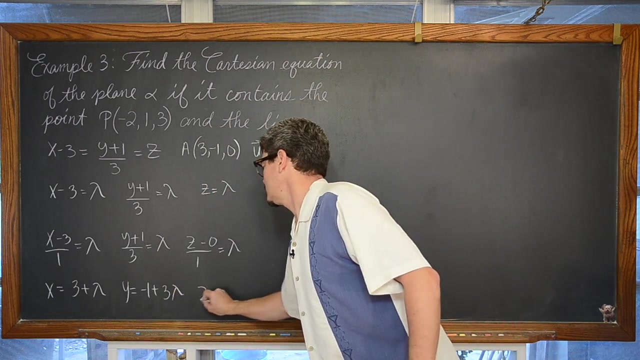 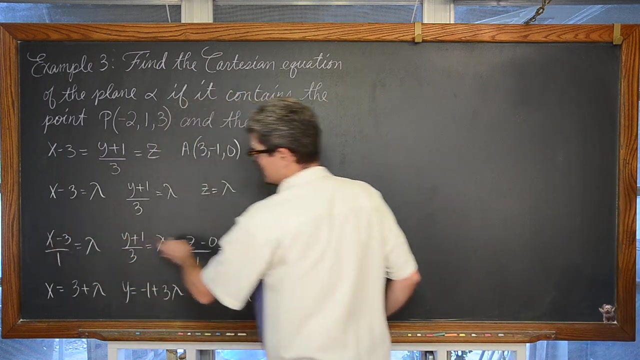 going to write. x is equal to three plus lambda. Coming down here, multiplying by three and subtracting by one, we have y is equal to negative. one plus three lambda, We have z is equal to zero plus lambda. So however you look at it, whether it is moving in towards, 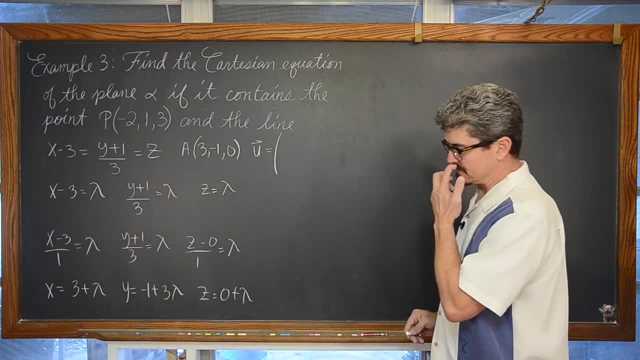 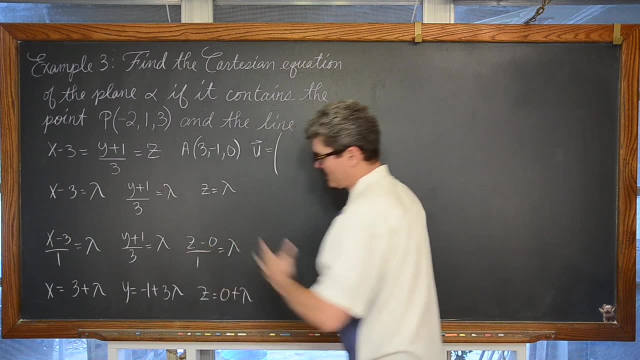 writing this in this middle step of the equation, or whether it is moving in towards the middle step of going into our parametric equations or just solving each of these for x, y and z, which, honestly, is better now that I am saying this, But we can see that point again. 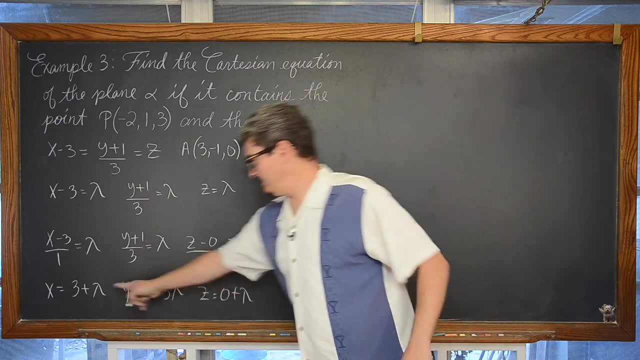 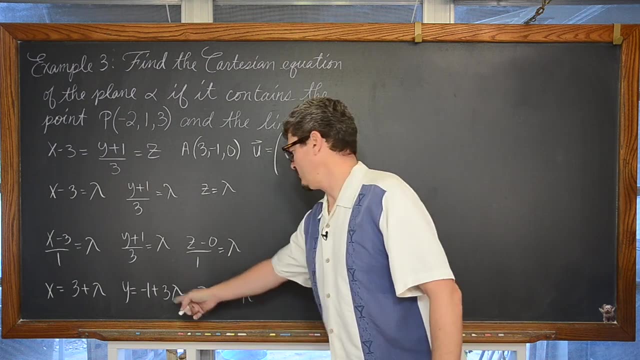 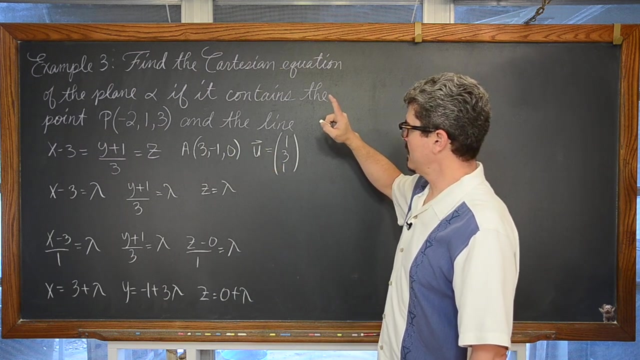 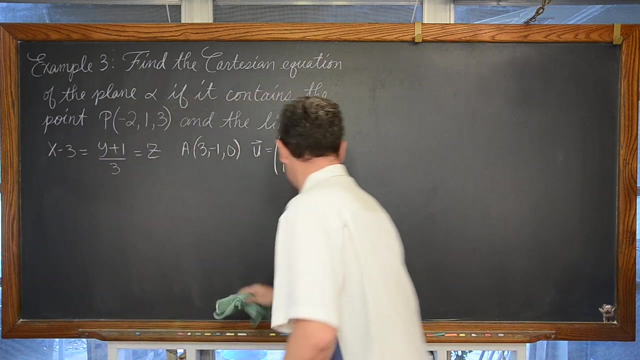 of three, negative one, zero here, And lambda is that scalar multiple of our gradient or directional vector, which is going to be one, three and one. So now we know a point and a direction. Ok, So it gave me a second to check my answer when my wonderful wife was answering the phone. 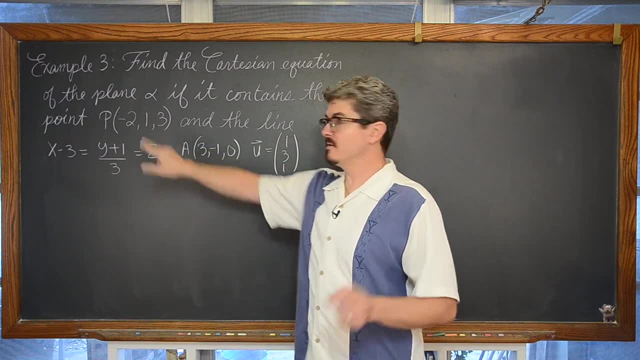 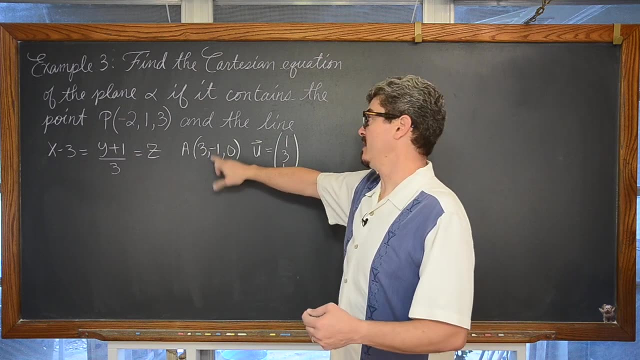 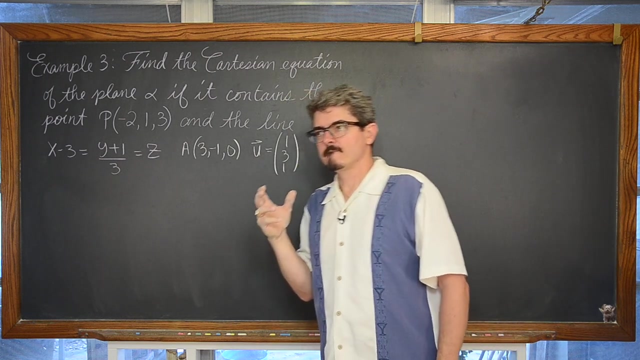 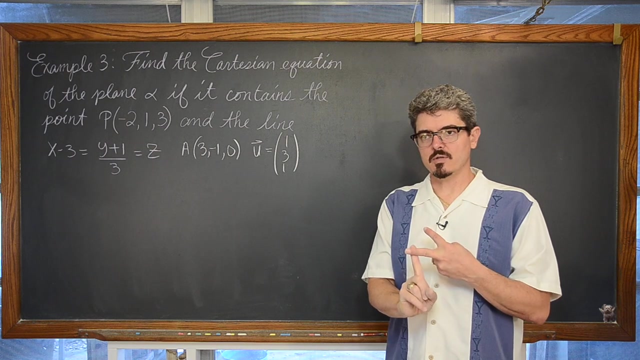 We now know for this plane alpha, one point that is on the plane, and we have this other point, which is also on the plane, because the plane contains the line and we have a direction vector. Well, whether we are going to use a normal vector or an equation or the just, 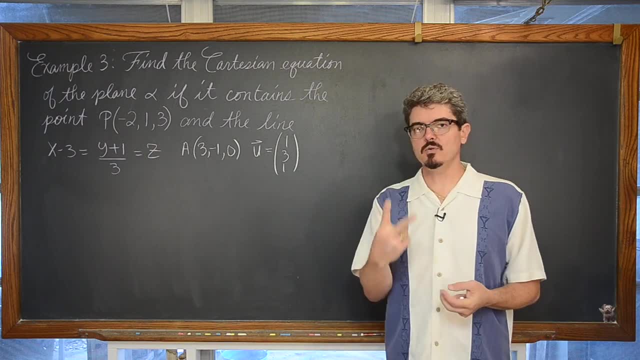 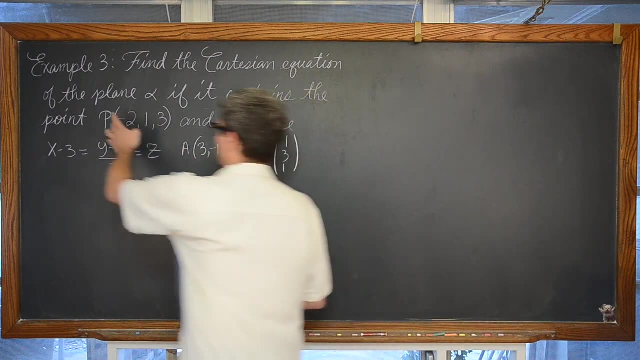 regular sort of vector form for the equation of a plane. we need two non-collinear vectors, And right now we only have one sort of gradient or directional vector for our plane, so we need another one. Well, we have that. We have two points that are in the plane, So we can. 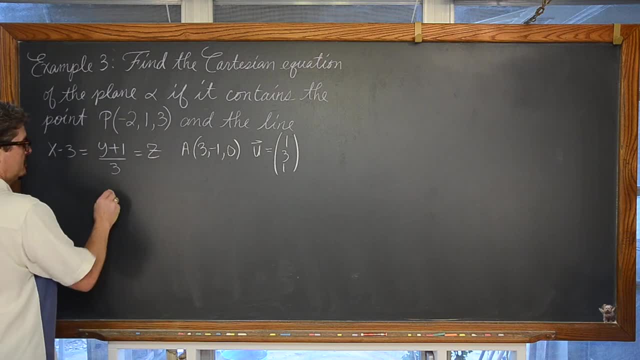 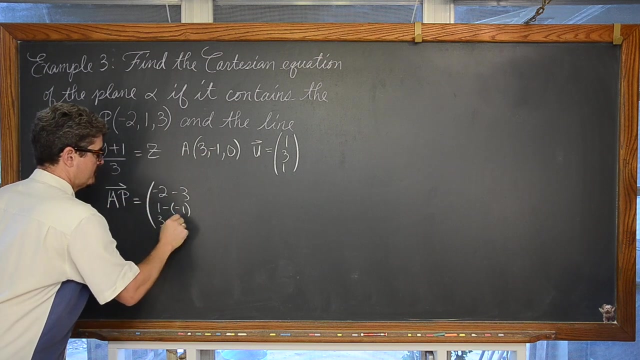 find vector AP, which is going to be terminal minus initial negative two minus three, one minus negative one and three minus zero, And so we have: vector AP is equal to negative five, two and three. So we have a point and 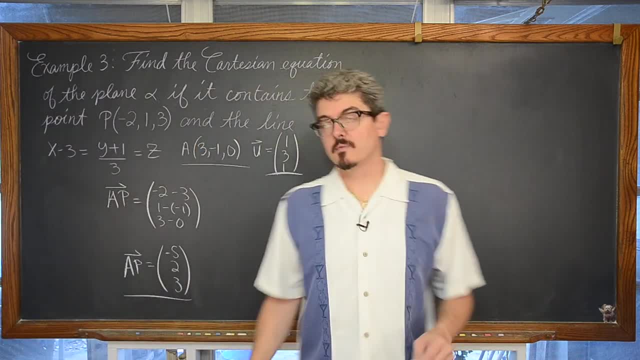 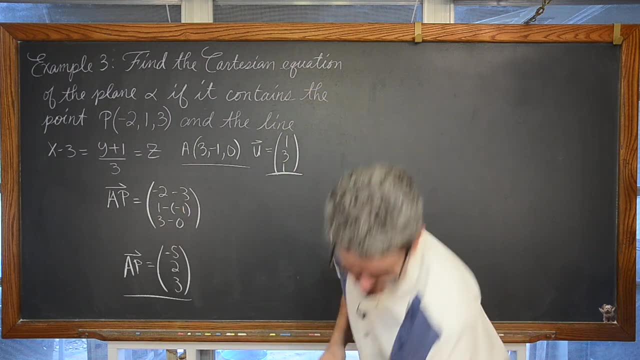 we have two non-collinear directional vectors that are together the gradient of this plane, And these are not scalar multiples of each other, so they are not parallel. Thus they wouldn't be useful. Now I just want to make sure that I haven't. 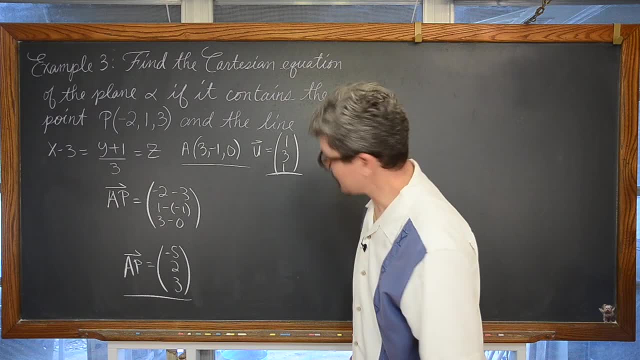 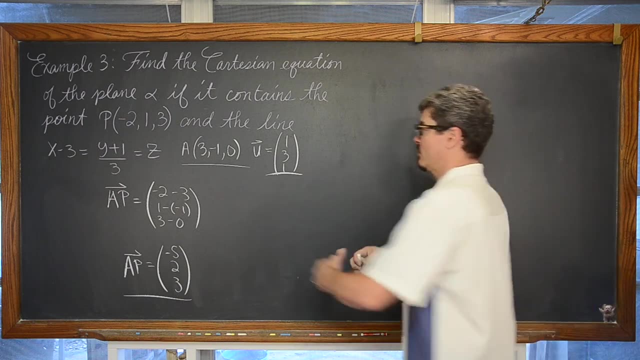 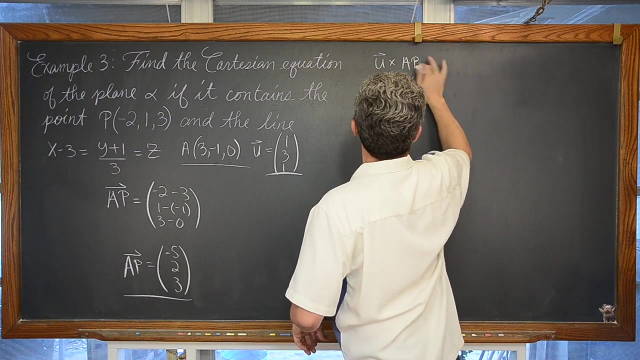 I wrote an incorrect number because I did some mental math incorrectly. Now we are going to find the equation of this plane by going through the normal vectors, which we are going to do. the cross product between U and AP which is going to be found, I will have 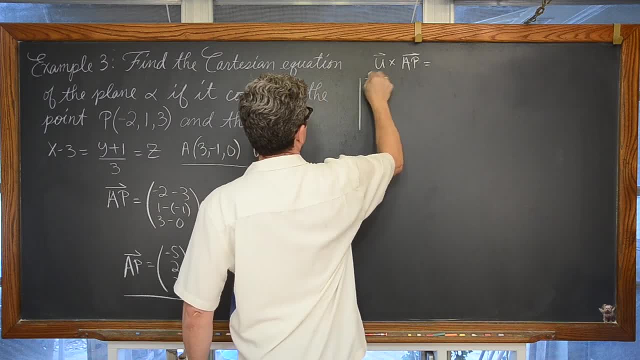 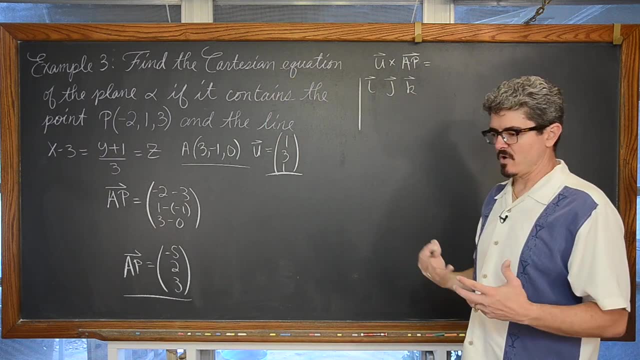 the answer up there in a second. by setting up a three by three matrix You might have noticed some patterns that you can use to find the cross product vector quicker. I just keep showing this process in case your teacher wants some really formal work and see that. 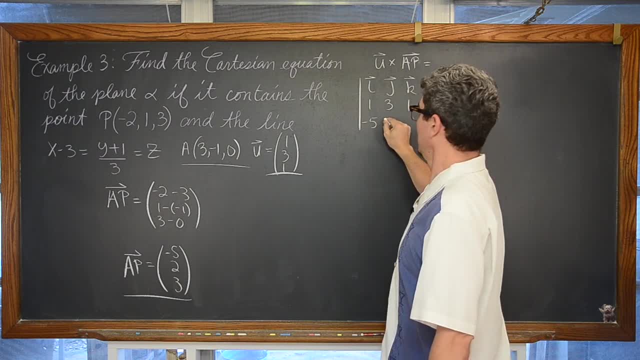 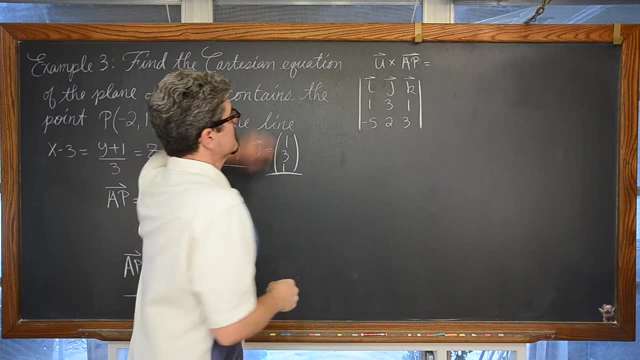 you actually know what is going on, not that you just recognize some pattern and sort of short cutting this process, But do whatever your teacher is happy with. This is going to be. we want the determinant. this is going to be equal to the determinant of this. 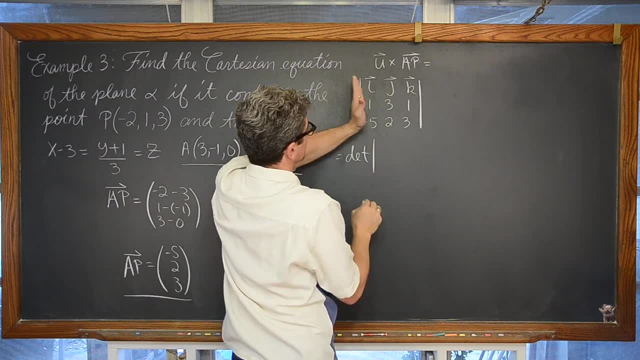 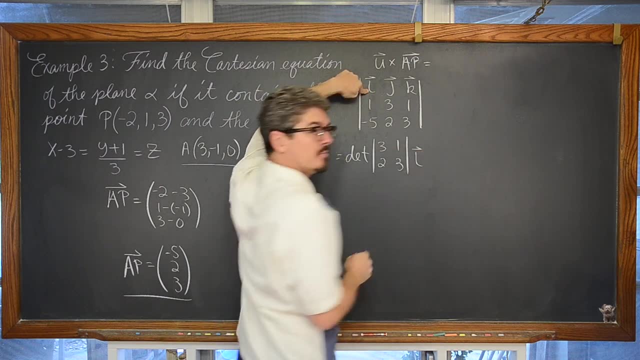 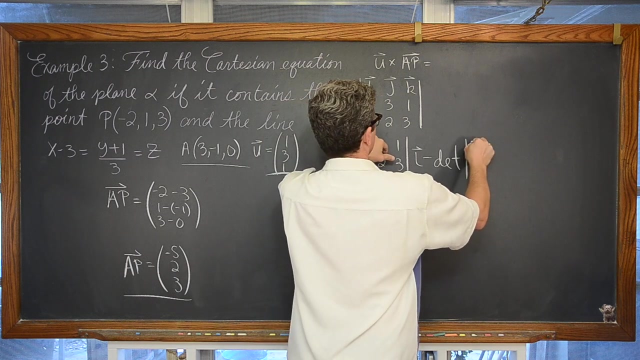 three by three matrix. So again Row, Row, Column and row that contains the i. taken out, That is going to be a coefficient of our i component minus the determinant. Take out the column and row that has again the j Vector, j component Plus the determinant of the two by two matrix. when you take out. 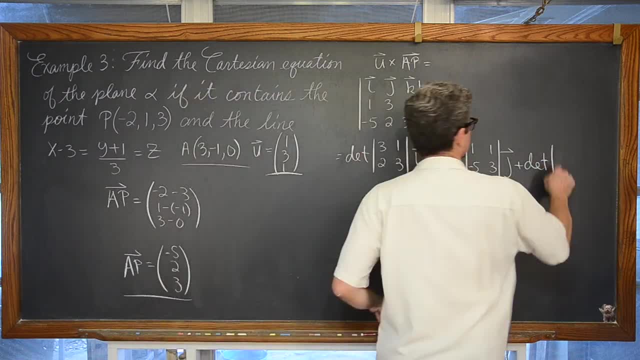 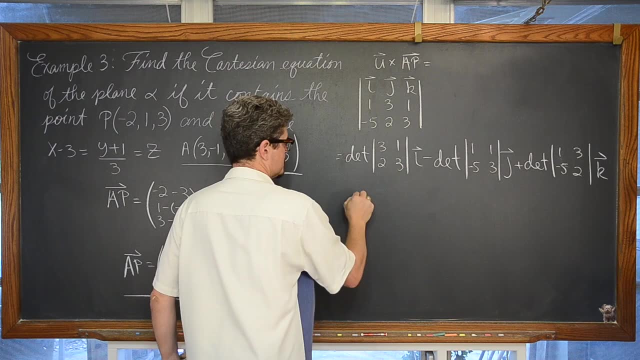 the column and row that has the vector component k. One last time, because this is the last example. Work out these little two by two determinants. We have nine minus two. We are given four divided by nine Minus three divided by 15.. This is going to. 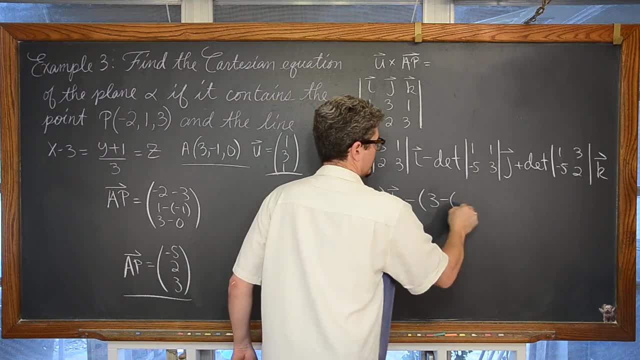 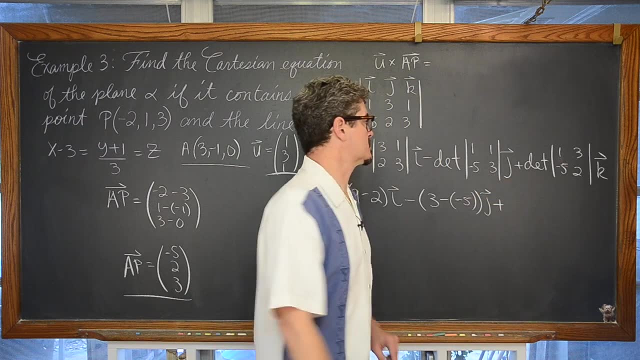 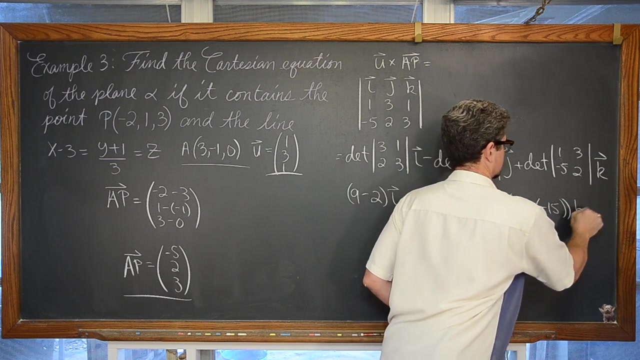 be our về i. We're going to divide that by one, So we're not going to have to fill this in, because we already had our lower power, 28. and there's the last room, which is not the two by three matrix we had as a requirement, for which is exactly what we wanted. We're going to dig this out, tylko got p resonant. So this is an indefinite number of ec�ömans. This is not just the two by two matrix, It is equal to 20.. We're going to call that. we have to note again: this is a predictor always, which is: 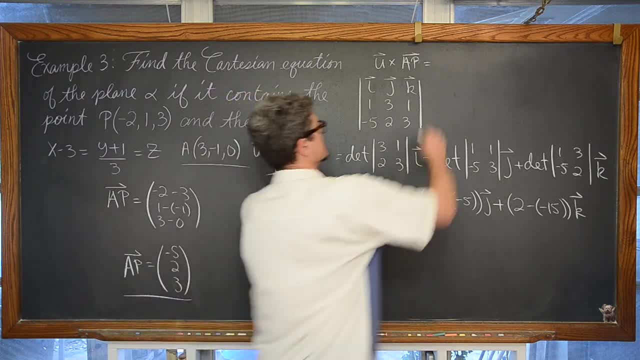 first to the класс plus the epsilon variance, complete Bahamian. So this is 280 plus 25. that will be our component for vector j. That will be our component for Vector J plus the determinant of this Column component form. 9 minus 2 is 7. 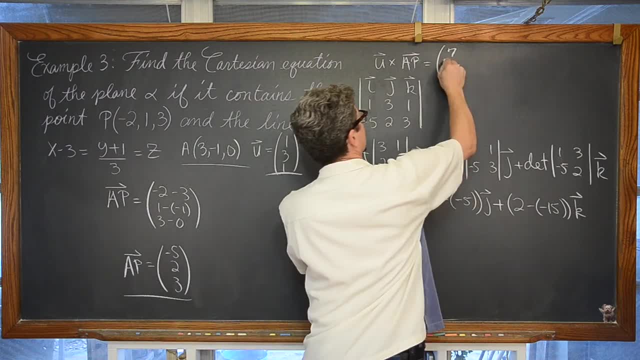 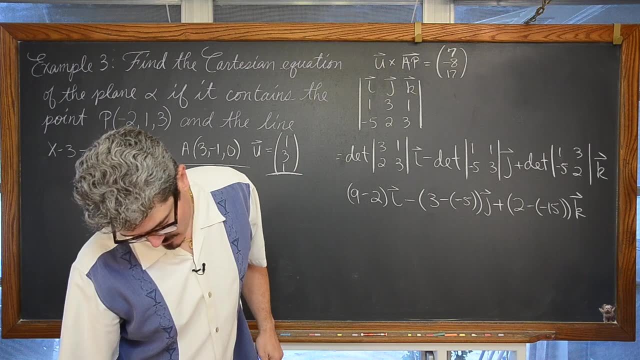 We've got 3 plus 5, which is 8, but it's got a negative out here, so negative 8 and 2 plus 15 and 17. Double check one more time, just so. we're good for the camera using that normal vector. 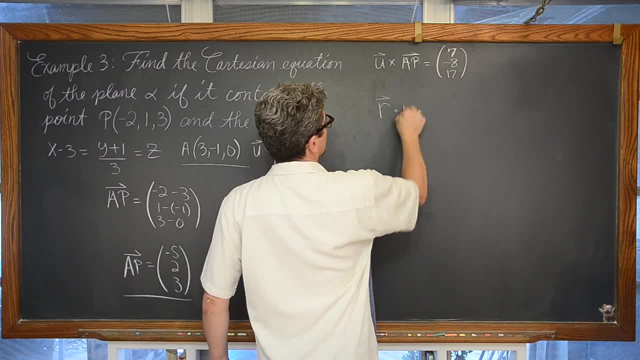 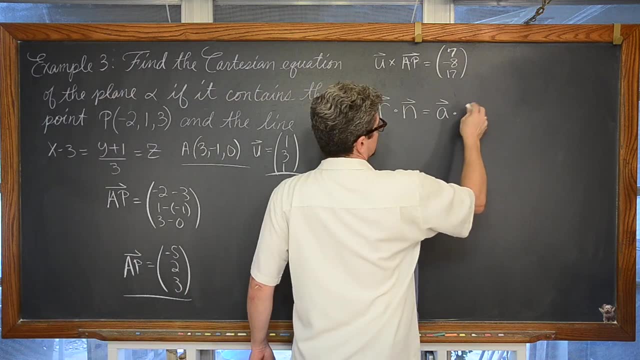 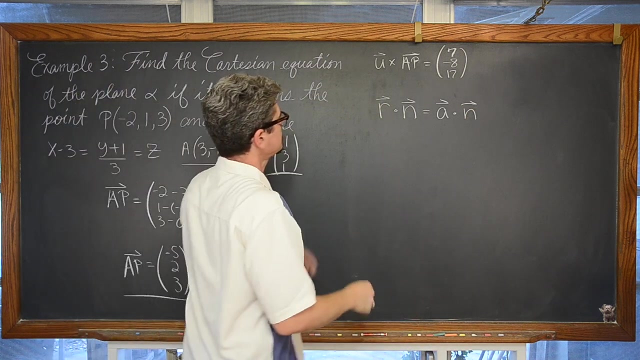 We're going to fill in this formula: vector r dotted with our normal vector equals some position vector for a known point on the plane, Taking that scalar product or dot product with that normal vector. and we have, And we do want this in Cartesian format. so when I go ahead and take the vector r and replace it with that, 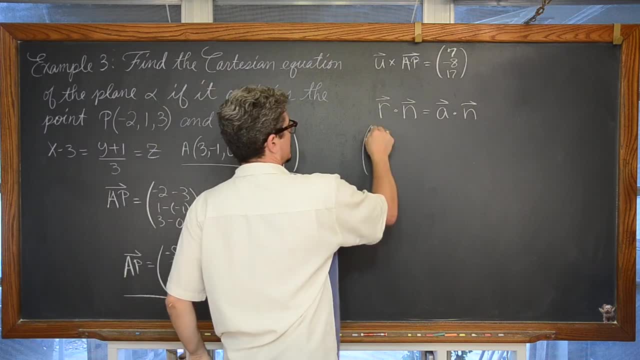 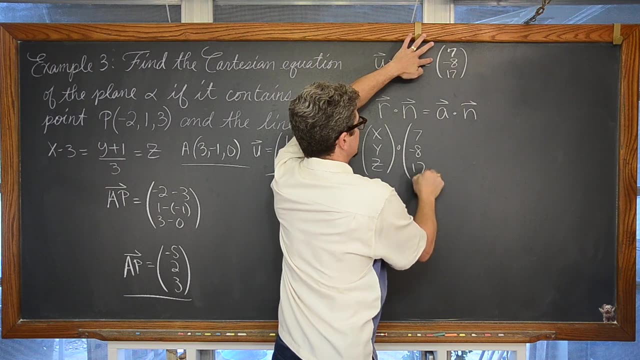 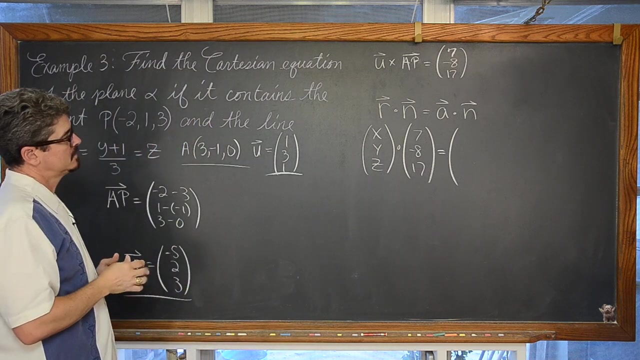 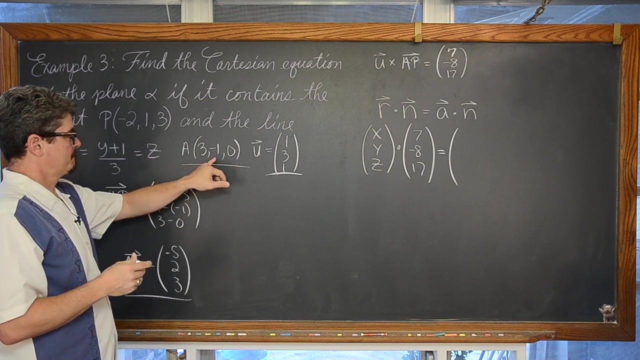 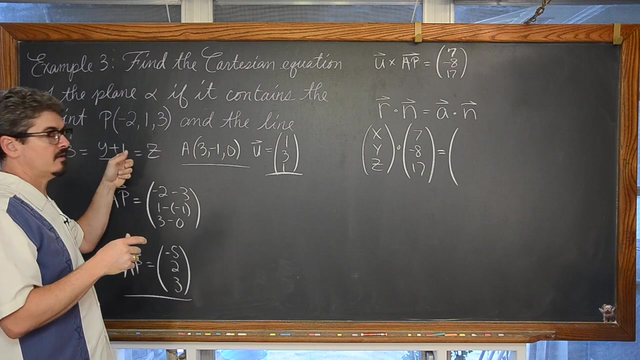 The component form of x, just x, y and z, general point on the plane. Dot it with our normal vector 7 negative 8, 17. I'm going to use coordinate a. You know, we we can't do this problem without Understanding how to find the point in the direction, the gradient of this line. so it's really kind of not a great idea to use. 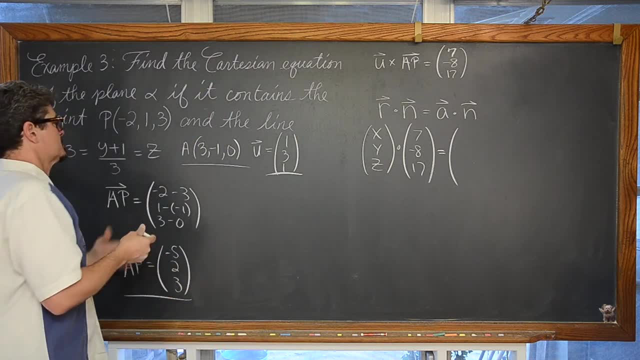 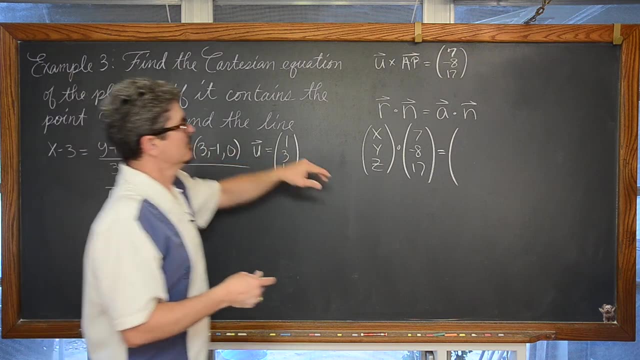 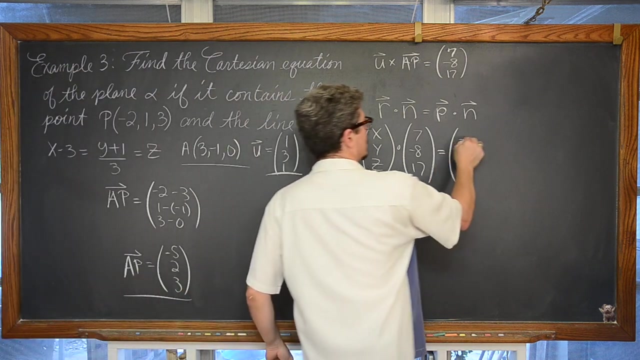 Information that you found yourself in your work, whenever possible, though this, this isn't right, the rest of our work isn't right, but You could use You know P Here and I could call this the position vector for coordinate P and have negative 2, 1 and 3. 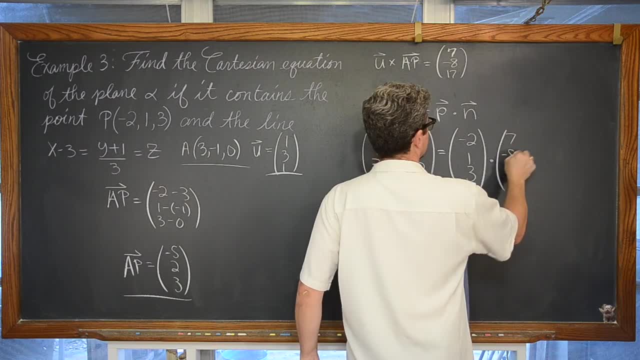 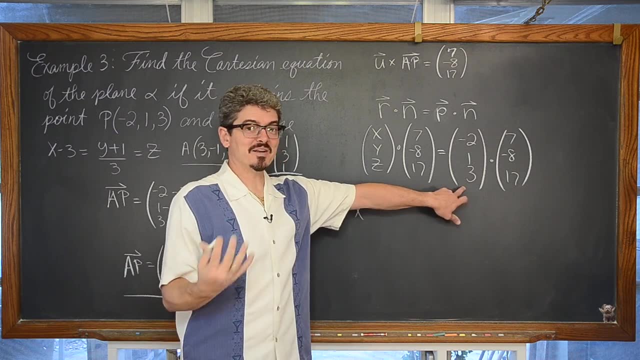 Dot that with our normal vector of 7 negative 8, 17, and we get 7x. By the way, I did not use Coordinate P in my notes. I use coordinate a. that I pulled from the line, but you'll see that we have the same answer. 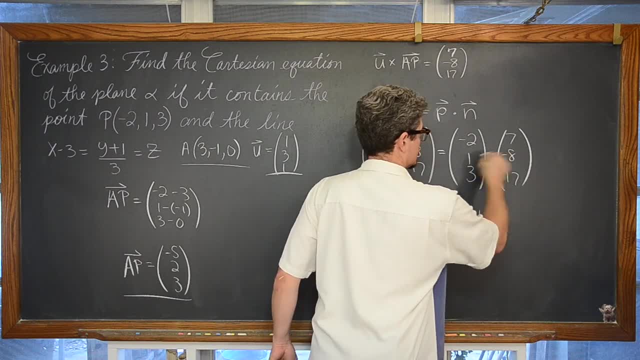 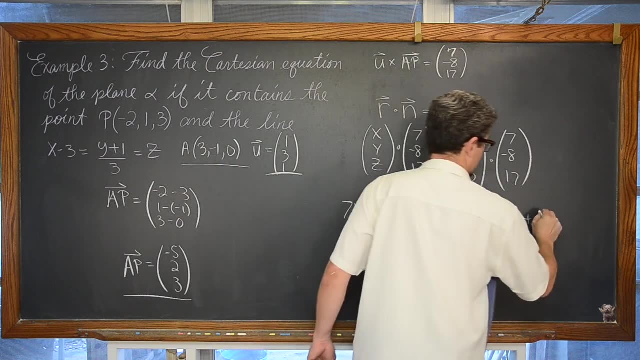 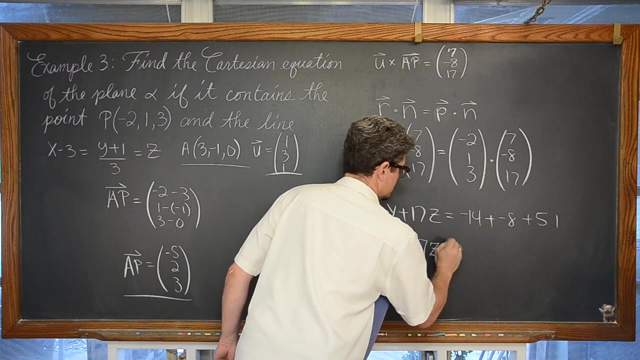 Negative 2 times. 7 is negative 14 plus 1 times negative. 8 is negative. 8 Plus we have 30 and 21 is 51. So we're looking at 7x minus 8y plus 17. Z is equal to negative.